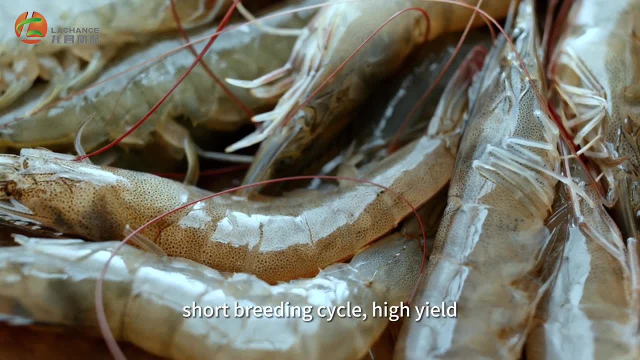 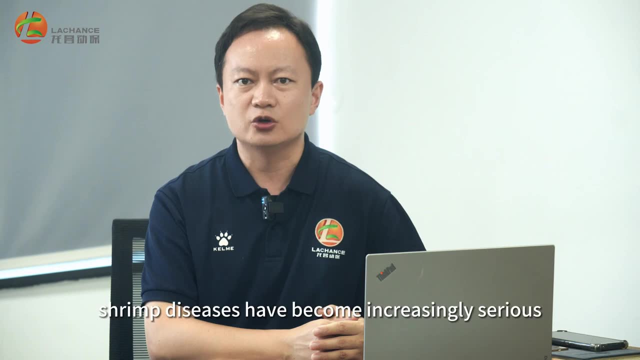 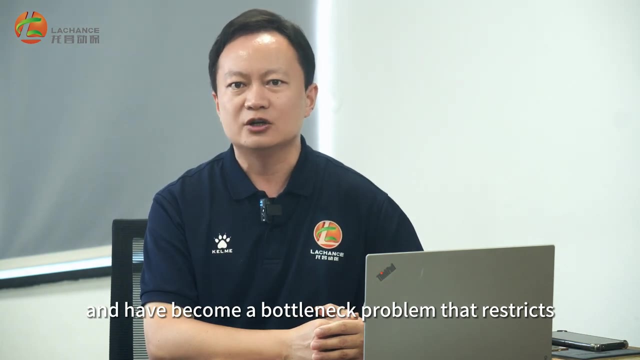 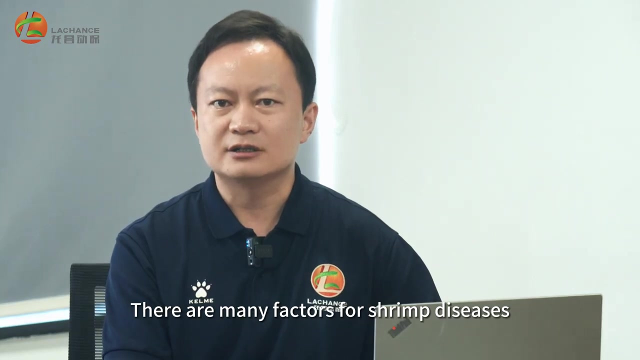 Shrimp has the advantage of faster growth, short breeding cycle, high yield and of various economic benefits. However, in recent years, shrimp disease has become increasingly serious and has become a bottleneck problem that restricts the development of the shrimp industry. The main causes of shrimp disease: there are many factors for shrimp disease, including environmental factors, nutritional factors, management factors and biological factors. 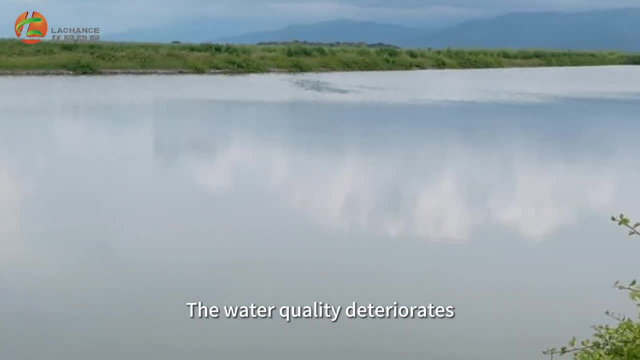 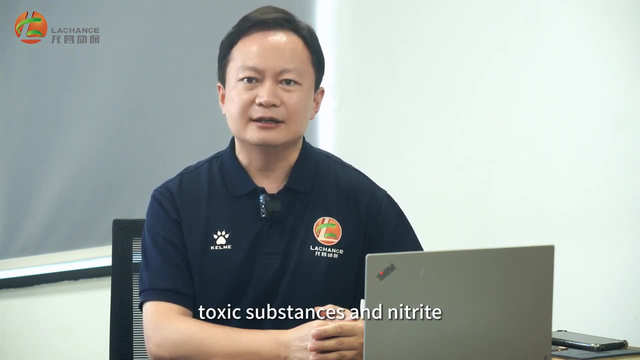 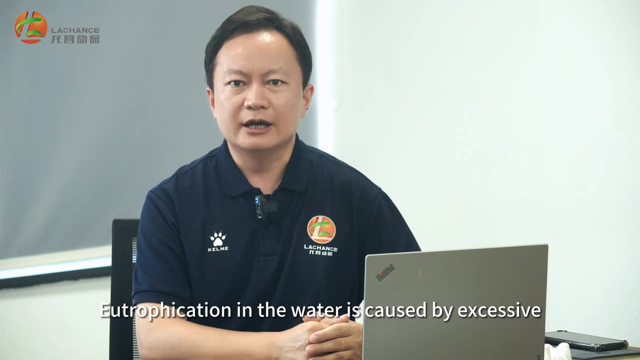 Environment is the first factor. The water quality deteriorates and many heavy metal ions, toxic substances and nitrites can directly harm and weaken the shrimp Eutrophication. Eutrophication in the water. Eutrophication in the water is caused by excessive residual feed, shrimp feces and organic pollution. 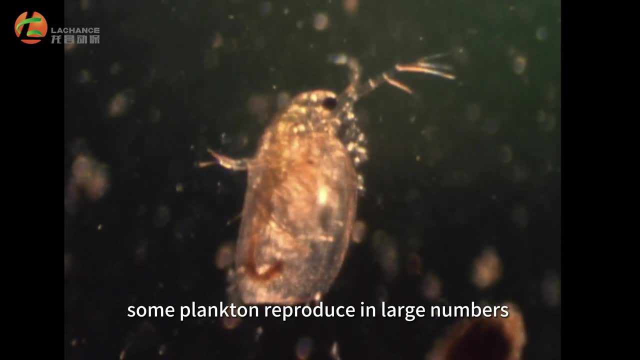 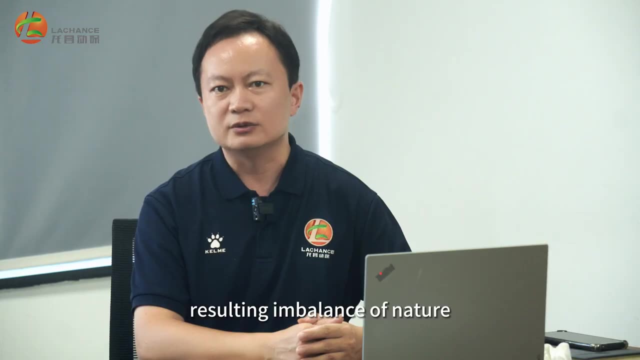 On the one hand, some plankton reproduce in large numbers without restriction, forming absolute advantageous species, resulting in balance of nature. In serious cases, red tide is formed, which further worsens the water quality. On the other hand, it promotes proliferation of harmful microorganisms. 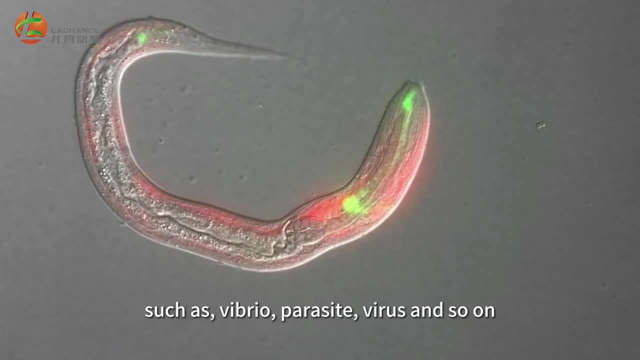 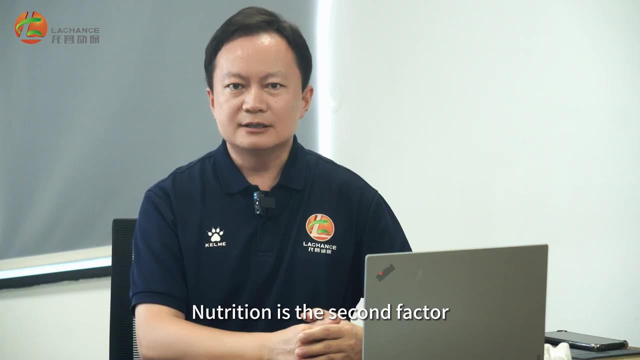 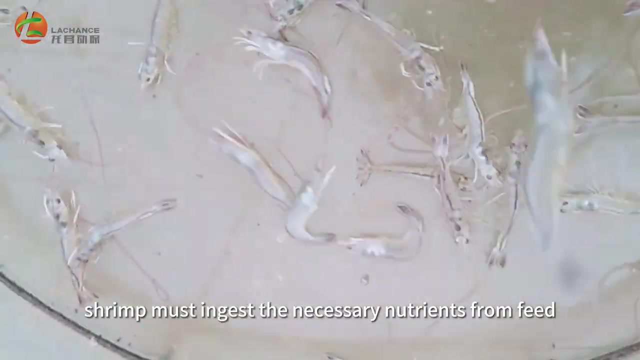 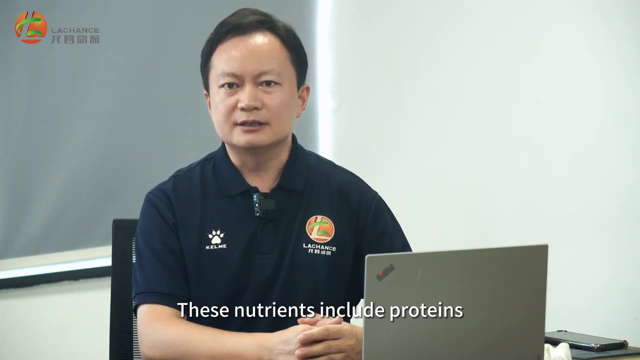 Such as viral parasites, viruses and so on, leading to the occurrence of various diseases. Nutrition is the second factor. In order to maintain life activities, growth and reproduction, shrimp must ingest the necessary nutrients from feed. These nutrients include proteins, lipids, carbohydrates, inorganic elements and vitamins. 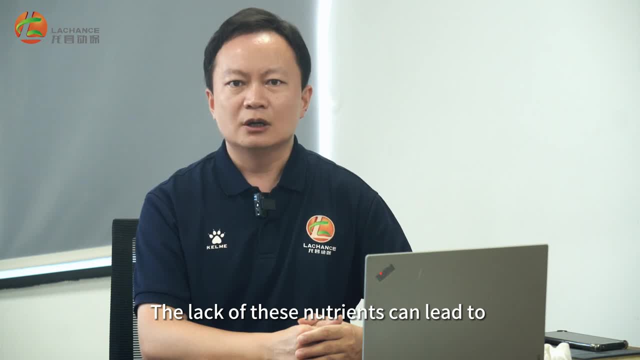 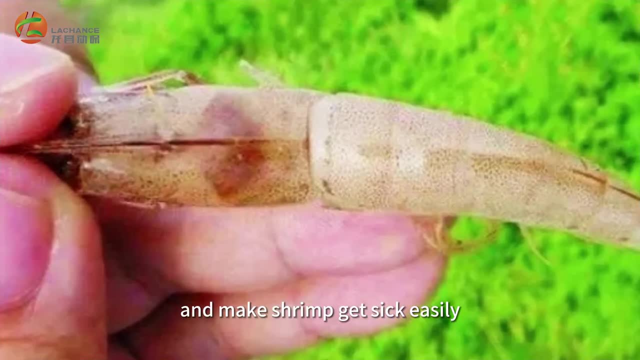 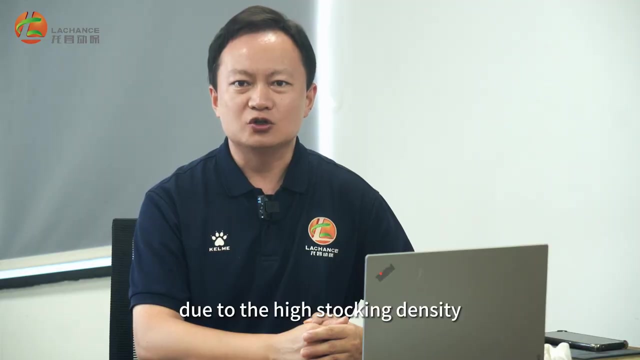 The lack of these nutrients can lead to corresponding deficiencies, reduce the shrimp's resistance and make shrimp get sick easily. Management is the third factor in the artificial cultivation of shrimp. due to the high stocking density, In addition to easily causing water quality deterioration, there are more opportunities for shrimp to contact with each other.